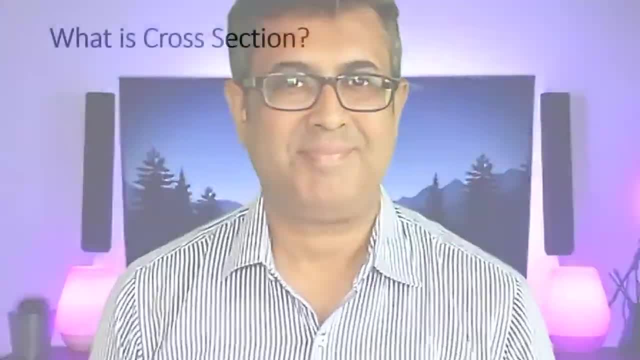 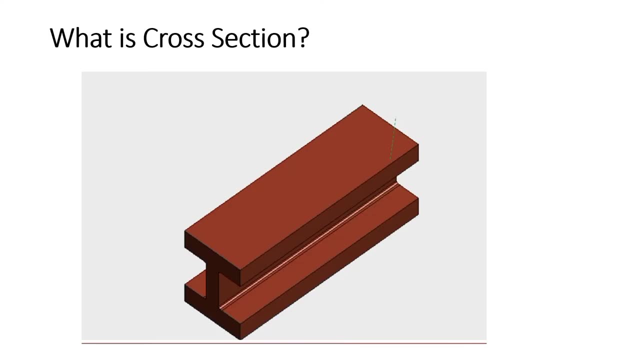 of learning structure analysis with STAT Pro. So what is a cross-sectional area? Imagine taking an I-shaped beam like this. Now imagine that you take a knife and cut this beam vertically downwards along the line AA. This is called taking a cross-section at AA or simply taking a section at AA. Now, when you cut the beam along this line, the 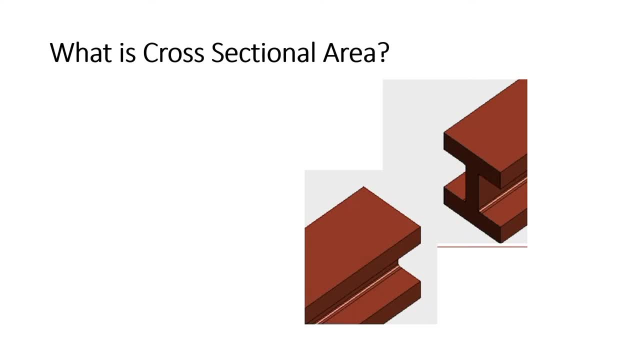 beam would be split into two halves along this line, AA and this particular plane depicted by the arrow sign. the area of this particular plane would be called the cross-sectional area. So what does it mean? So which area of this particular plane could be called the cross-sectional? 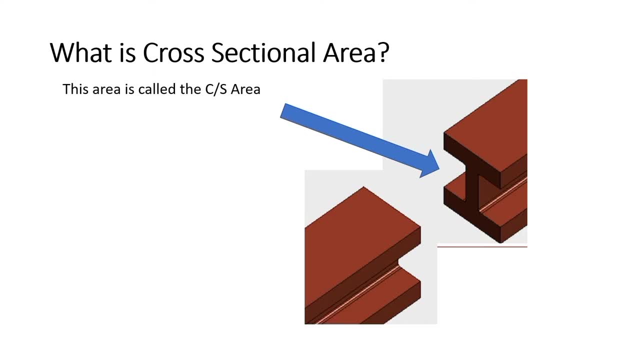 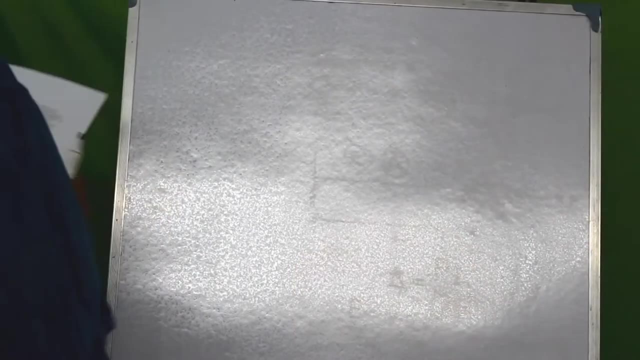 area. If you have a W14 by 873 American eye section, or the white friend section as you would call it, that would typically have the dimensions as shown on the screen. So how do you calculate a cross sectional area? Well, the members made of concrete usually. 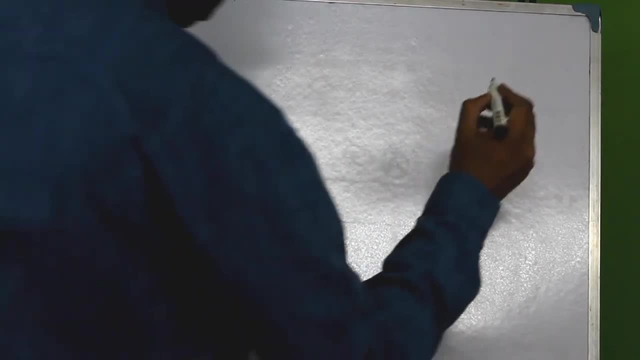 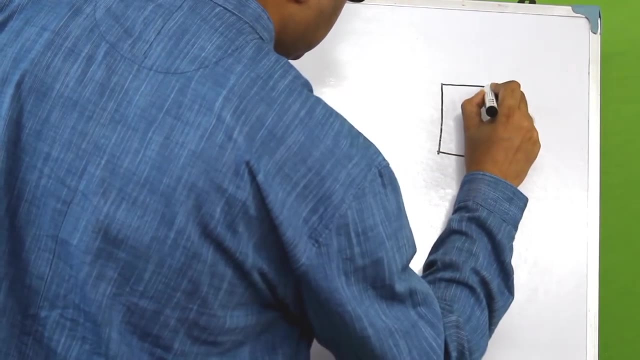 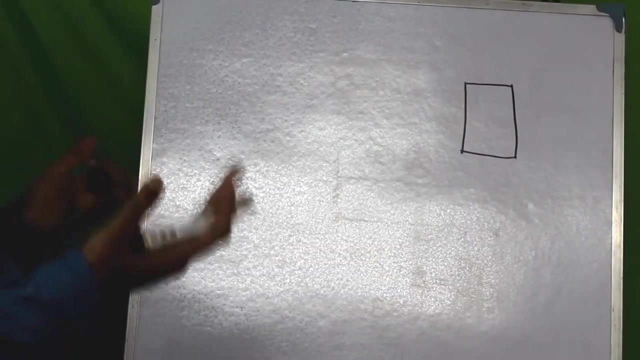 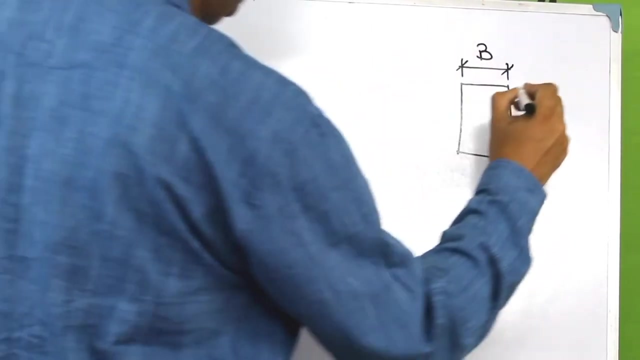 have a rectangular or a circular cross section, So a rectangular section looks like this. So, in case of a rectangular section, which is common, in case of when the material is concrete, let us consider the width of the section as b and the depth of the section. 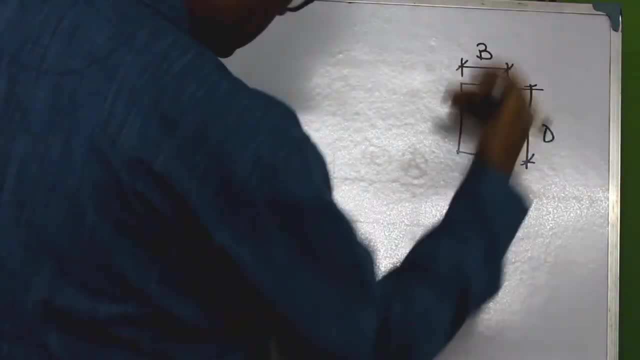 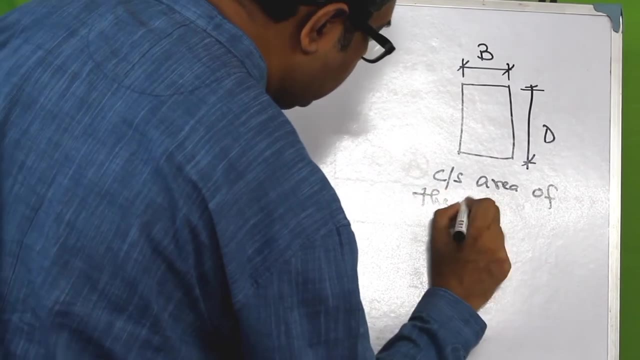 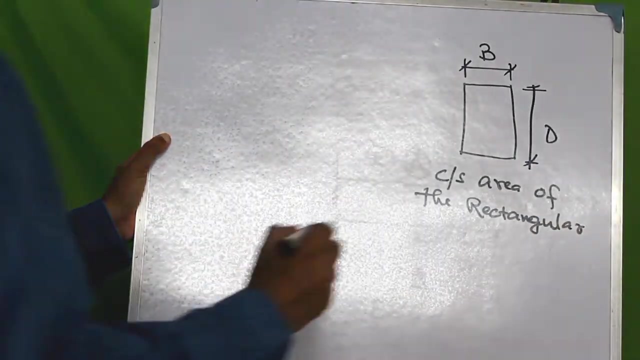 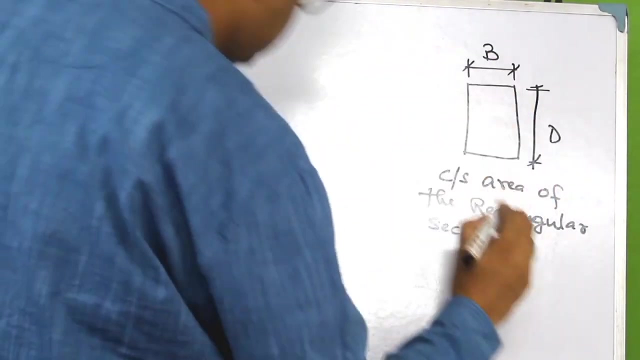 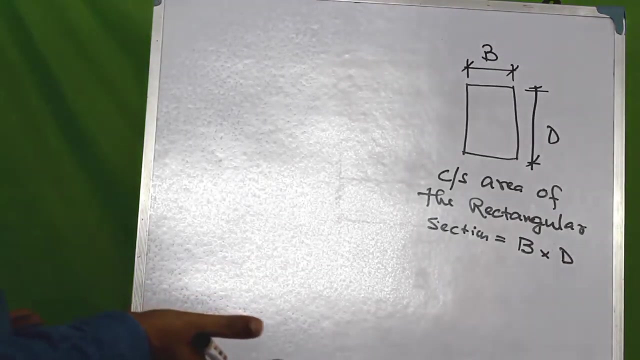 as d, Then the cross sectional area of this particular section is given by- and we have studied this in our primary schools- what is the cross sectional area of the rectangular section? So it is given by this width into this depth. So it would be b into d. So that's the cross sectional. 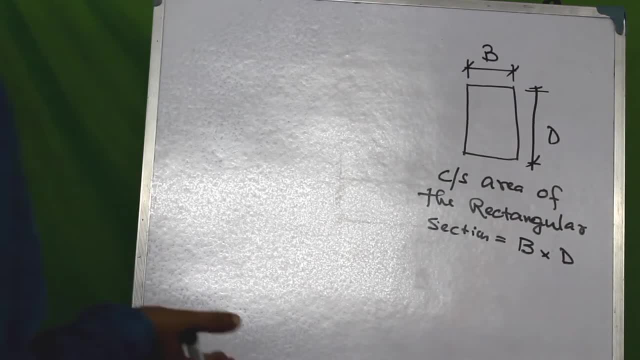 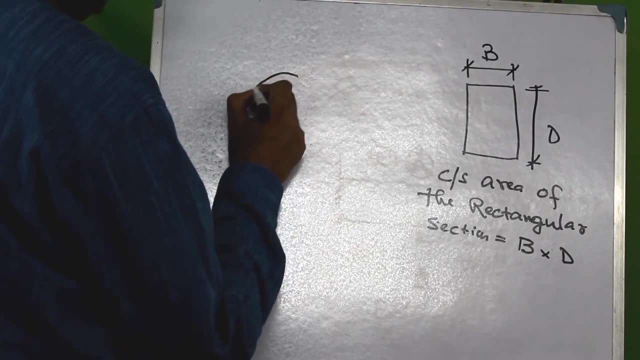 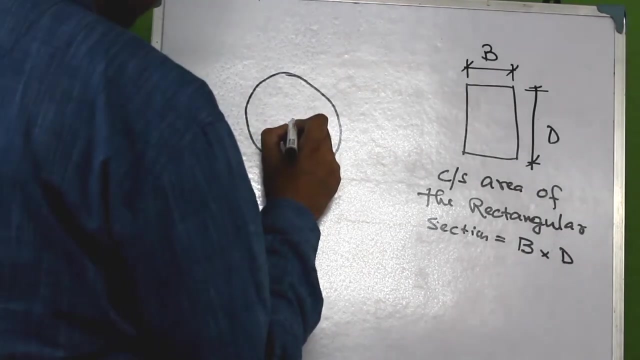 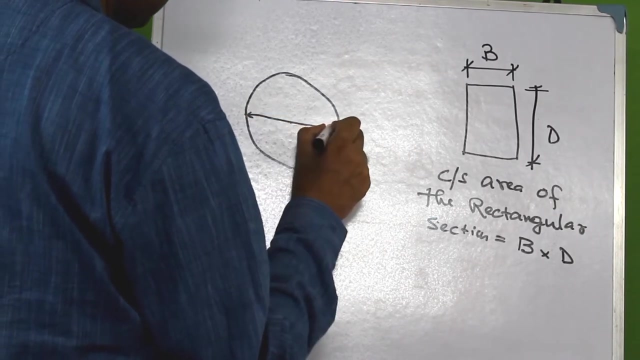 area. The other common type of cross section, in case the material is concrete, is a circular cross section And generally you would find columns having this type of cross section, short, critical section. Now, if this cross section, this circular cross section, has a diameter d, then the cross sectional area would be: 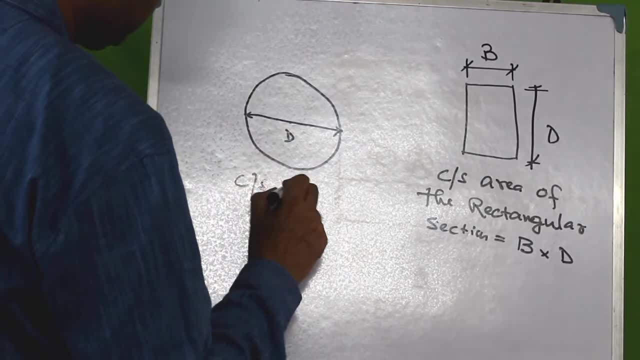 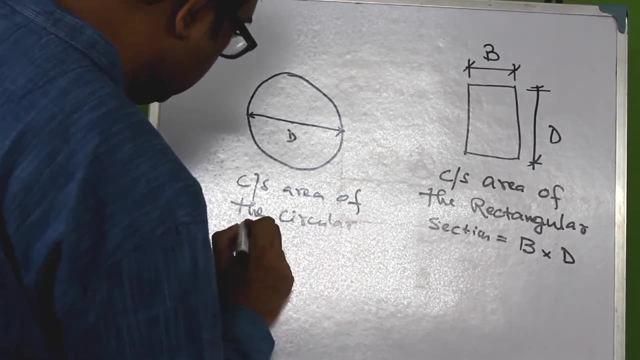 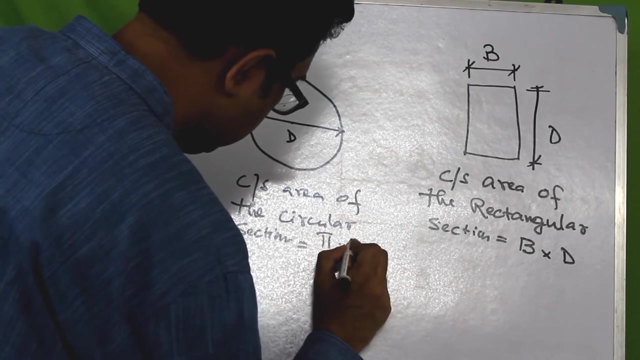 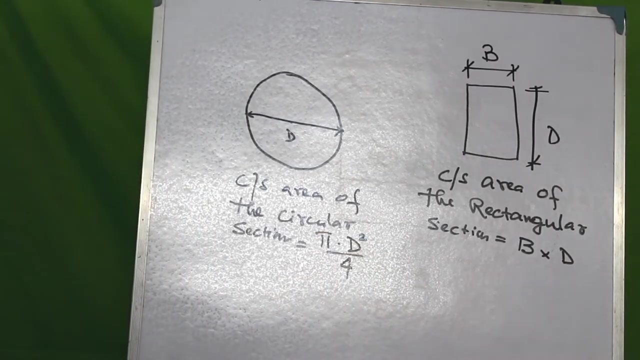 e to the length, Talen b, www, tanب b and b of the circular section is given by pi into d, which is the diameter squared by 4.. So this is the cross sectional area of a circular cross section. Now let us consider the cross. 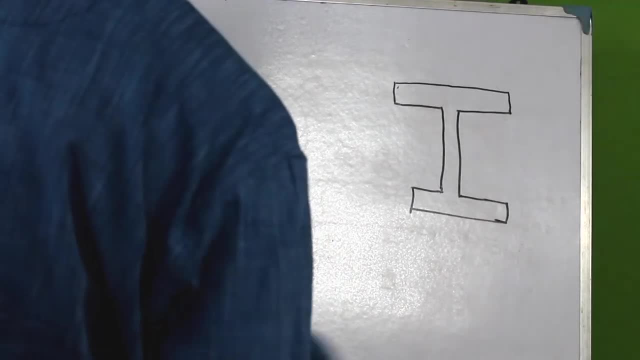 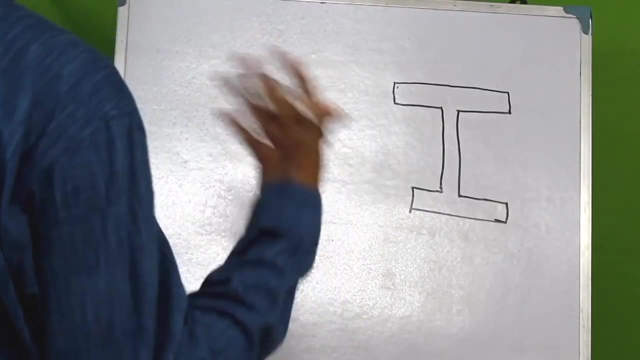 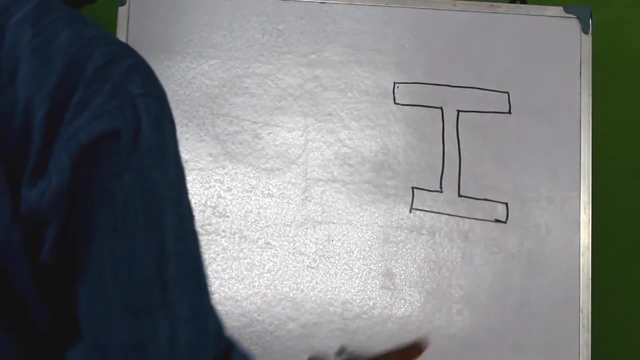 sectional area calculation for some common shapes. that relates to steel cross sections. so, or rather, the material that we are considering now is steel and the cross sectional shapes that are available with the steel material. So one of this shape is an I shape, which you can see on the screen. 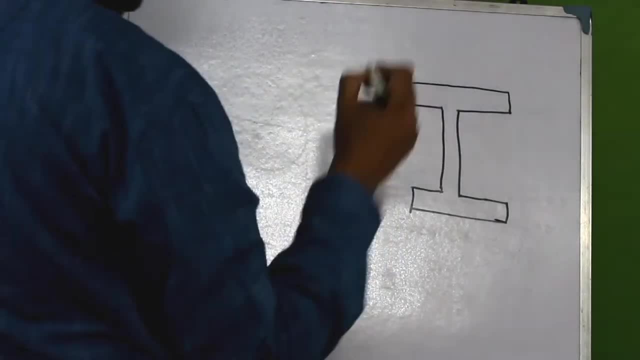 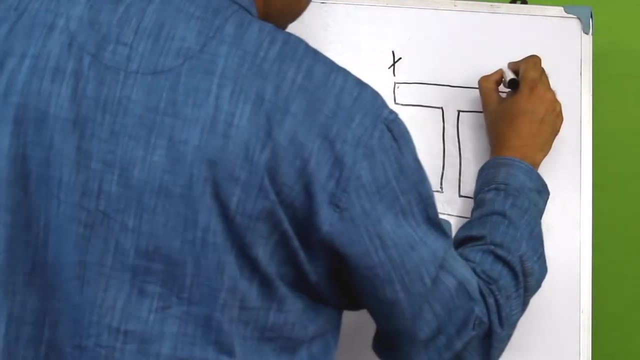 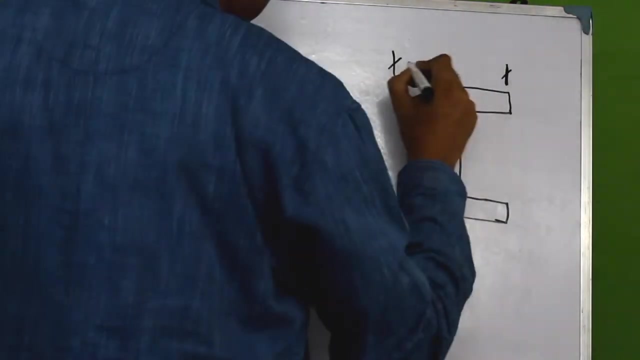 And let us represent the I shapes, the dimensions of the I shapes with the notations that are used in the STAD user table general sections. We will discuss more about user table general section as we proceed in the course, but for now let us consider the dimension representations. 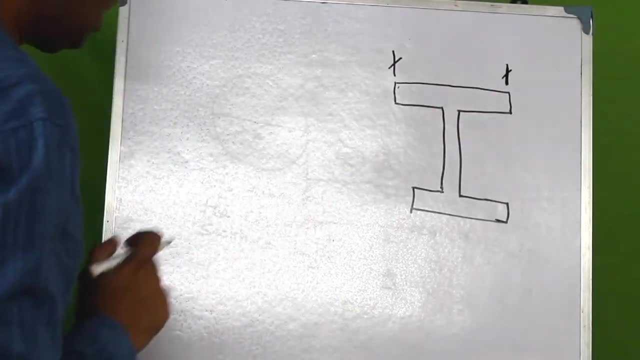 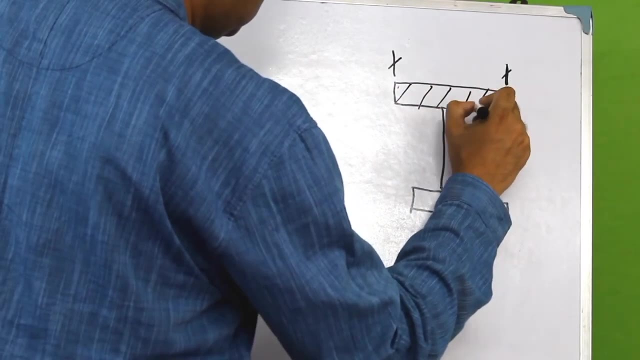 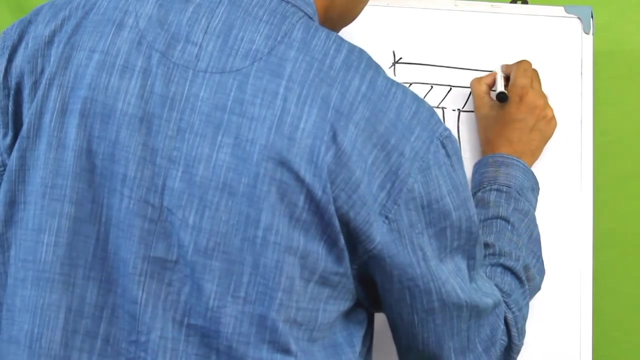 that are being used there to represent the various dimensions of the I section. Now this part of an I section is called the Top Flange, So the top rectangle and the width of the I flange. in STAD user table general section is represented. 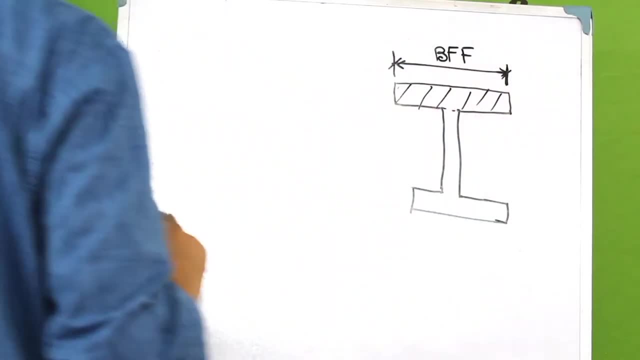 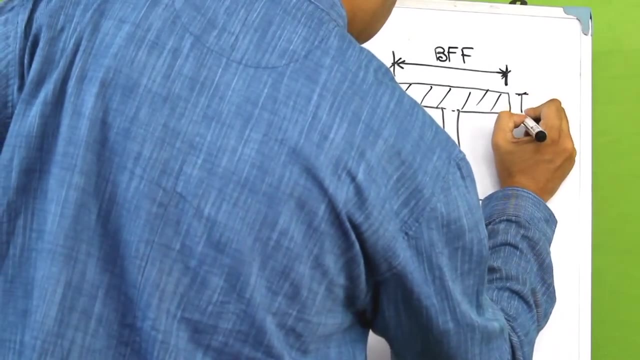 as BFF, which sort of represents the breadth of the flange, and then the thickness of the top flange is represented as h2.. So I divided that by hgf and this and the width of the i flange in STAD user table general. 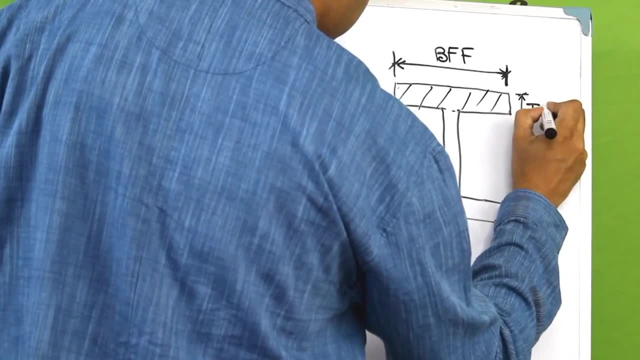 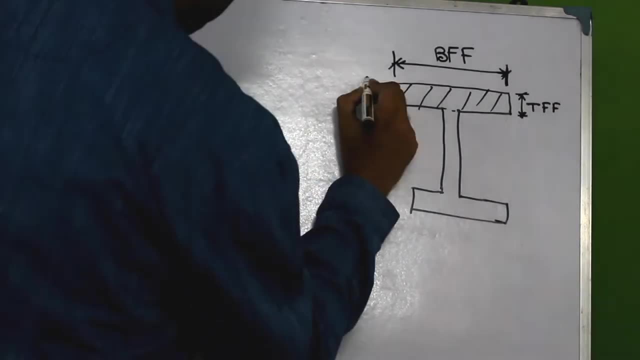 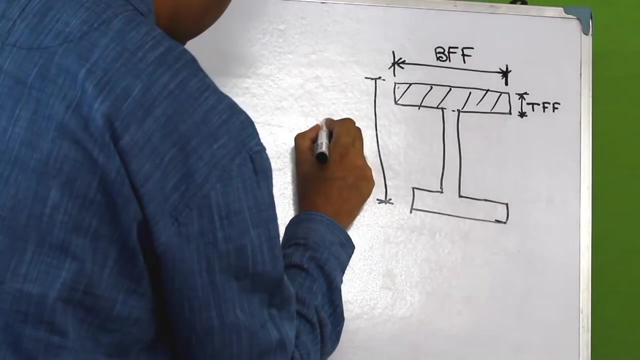 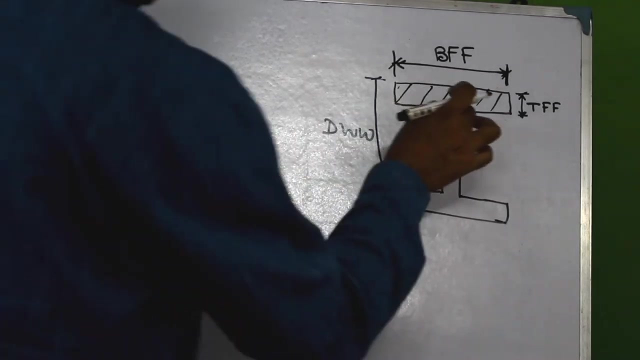 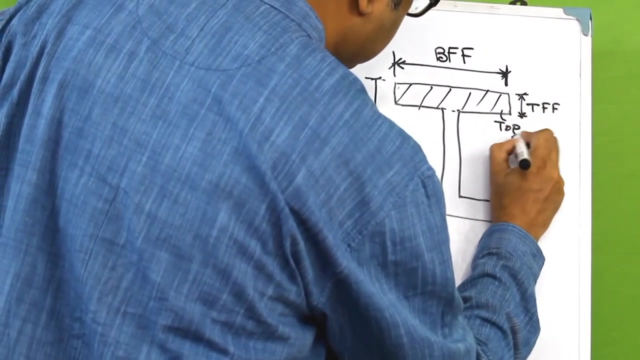 section is represented as bff. Ok, The total depth of the section, which is from the top of the top flange till the bottom of the bottom flange, is being represented as DWW. Then the thickness of this portion here. now this is called. see, this is the top flange. 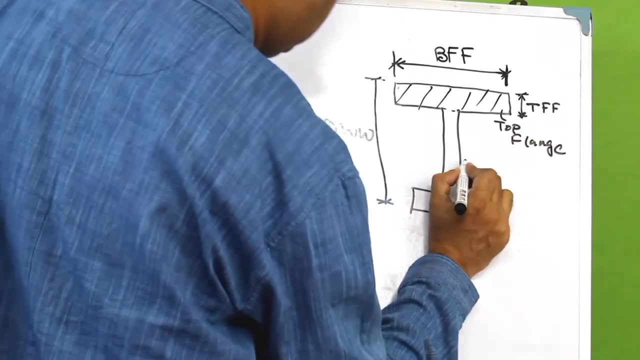 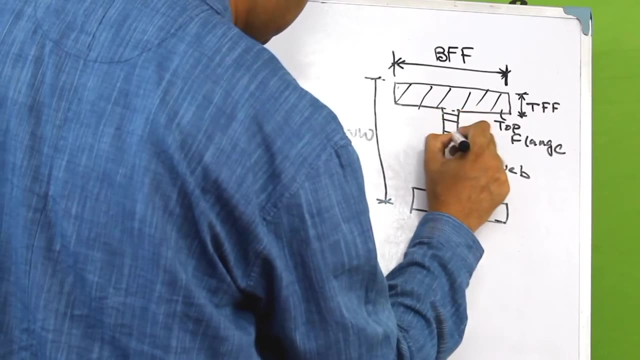 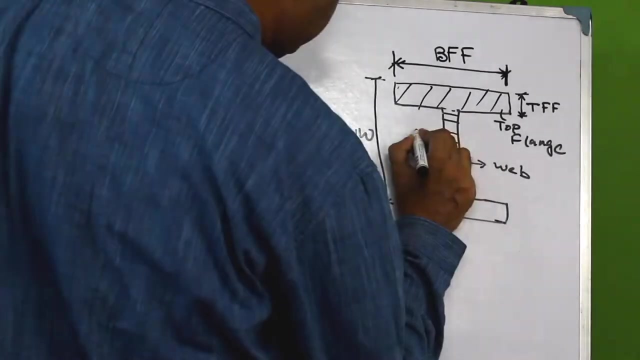 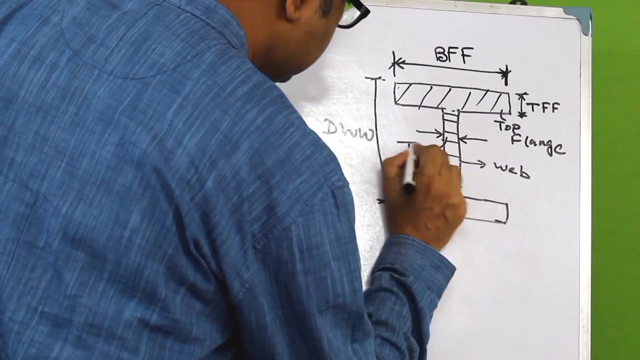 this is the top flange and this is the web of the section. okay, And so this would mean this section here. This is this rectangle here is called the web of the cross section, and the thickness of the web in STAP terminology in terms of user table general section is given as TWW. 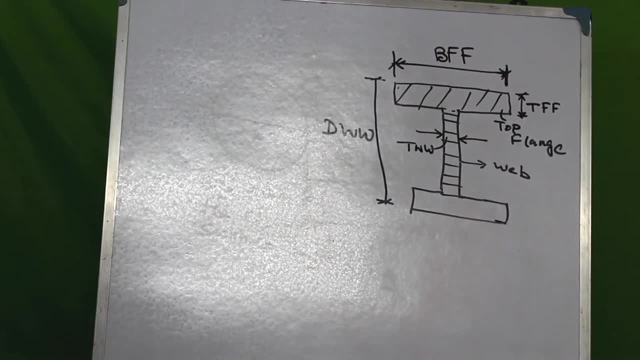 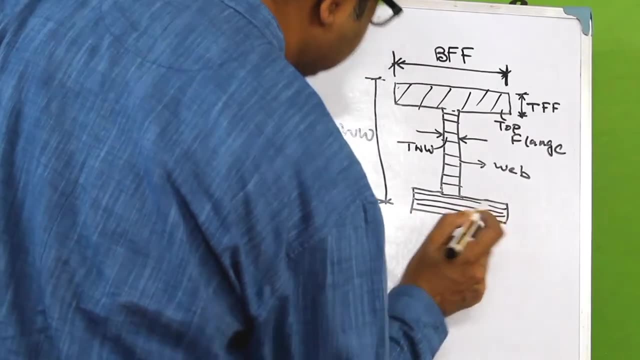 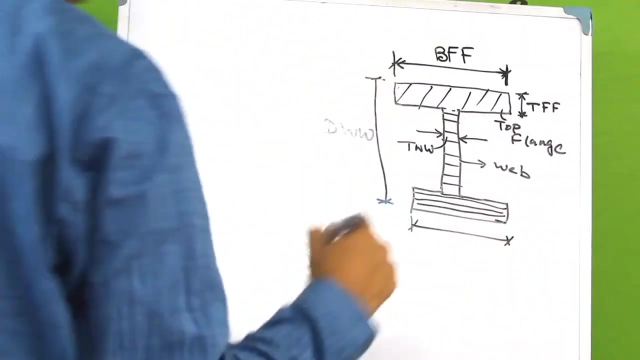 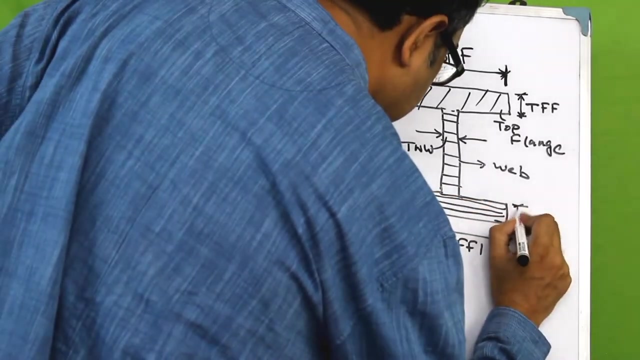 which would mean the thickness of the web. And finally, the last portion is called the bottom flange. okay, and this bottom flange is another rectangle and the dimensions can be represented. as for the width of the bottom flange, we can represent that as BFF1 and the thickness can be represented as TFF1.. 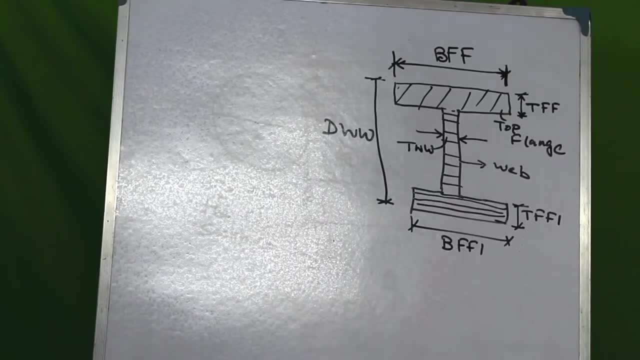 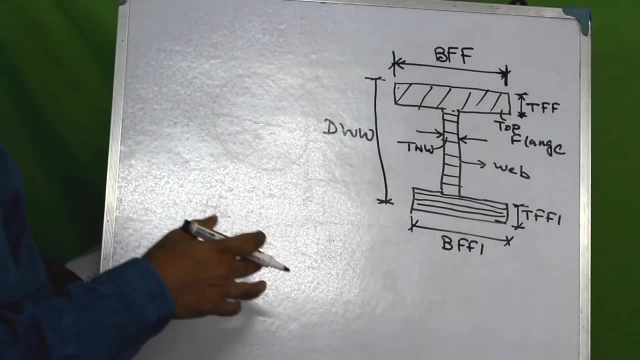 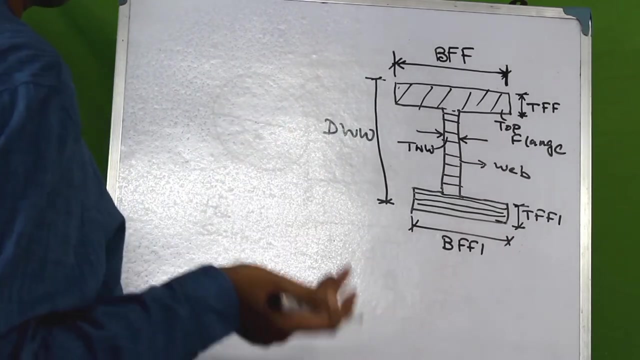 Now, how do we calculate the area? Okay, So the area of this section. so the area, the area of the cross section, would be nothing but the summation of the cross sectional areas of all these simple rectangles. right, And we already know what the cross sectional area of the rectangle is. 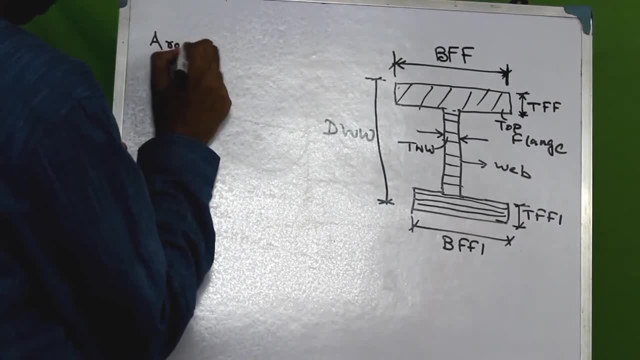 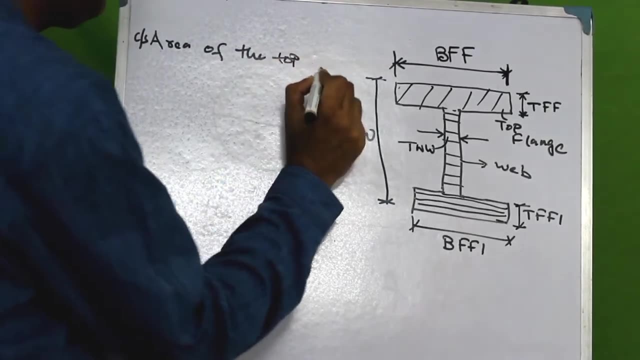 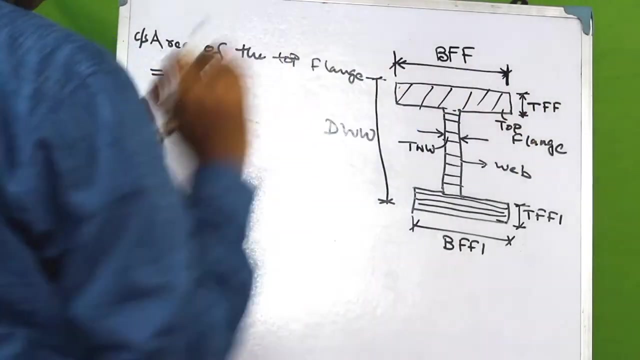 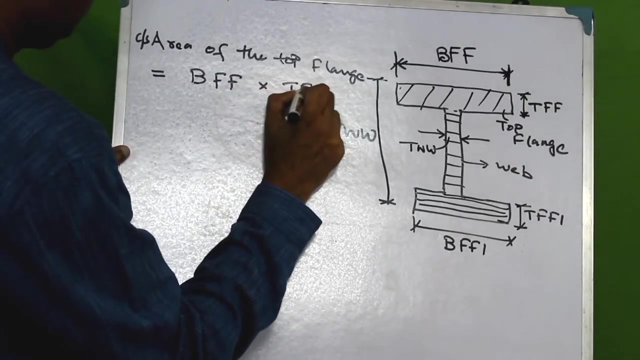 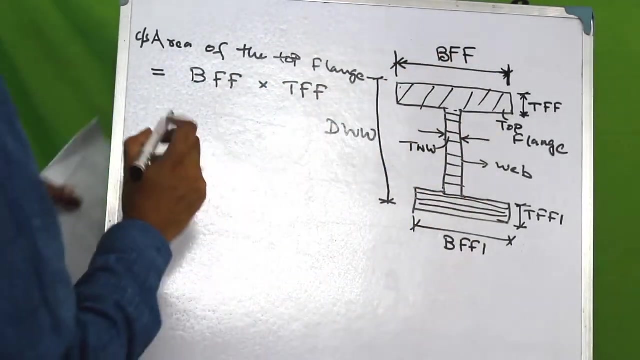 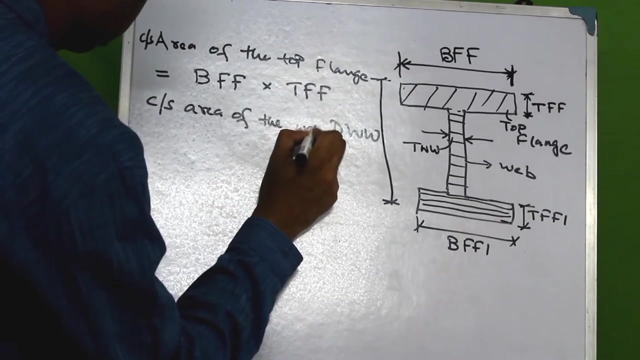 So the area of the top flange, the cross sectional area of the top flange, So the area of that of the cross sectional area would be equal to the width into the depth. so it would be BFF2, TFF. what would be the cross sectional? area of this web here. well, This is another rectangle, So it would be the depth of the web, which is Q, the width in the least depth of the web. Now, how do we determine the width in the least depth of the web? braid. 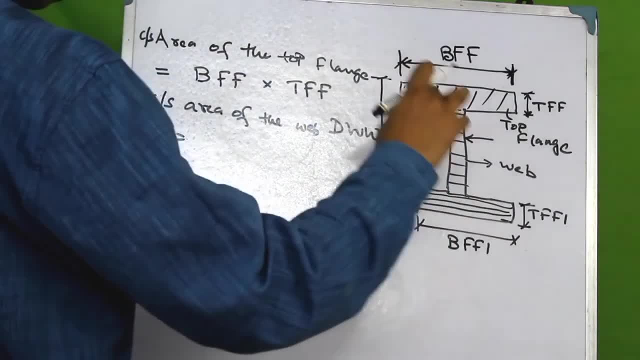 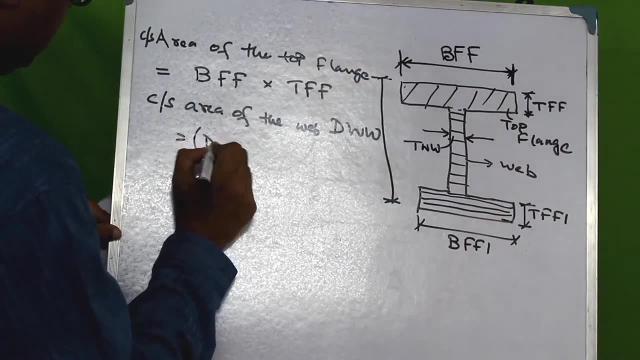 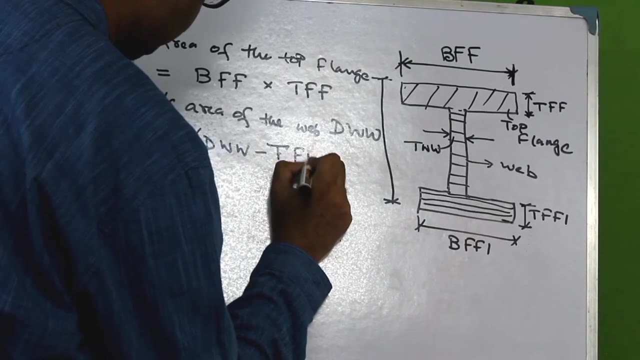 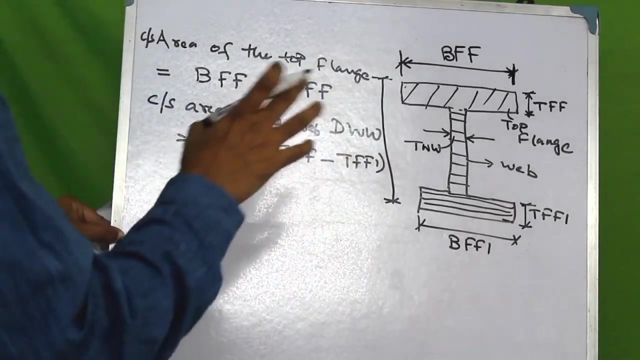 All right, which is the total depth minus the thickness of the top flange and the thickness of the bottom flange. so we'll have: this is the total depth minus thickness of the top flange, minus thickness of the bottom flange. this is, this would be, the depth of this, this section, and what would be the width of. 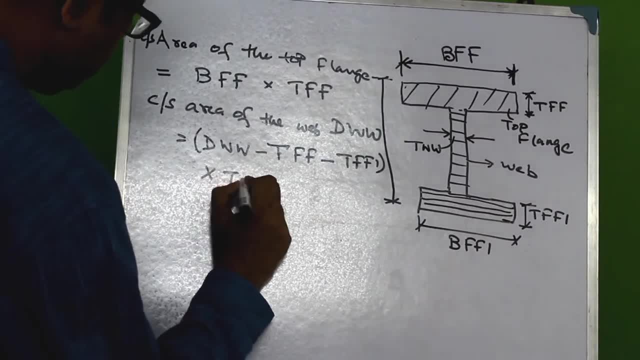 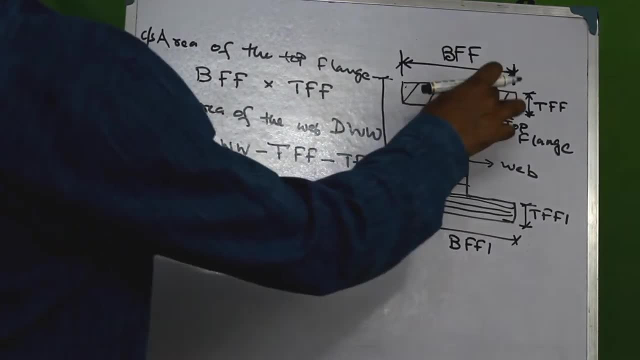 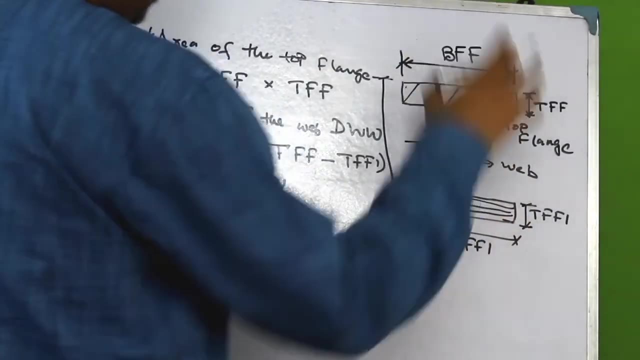 this section would be the thickness of the web, which would be TWW right. so this, multiplied by this, would give the cross-sectional area of this web. and finally, we have one more component of this particular section, which is the bottom flange. so let us find the cross-sectional. 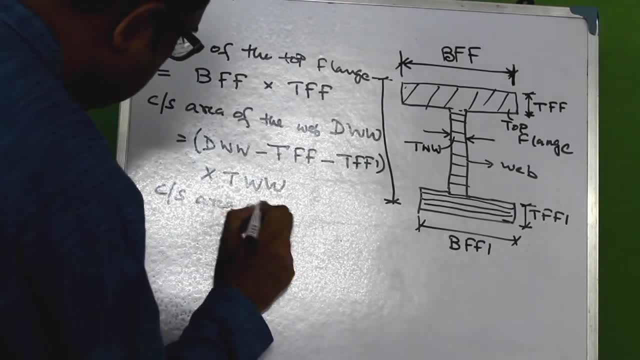 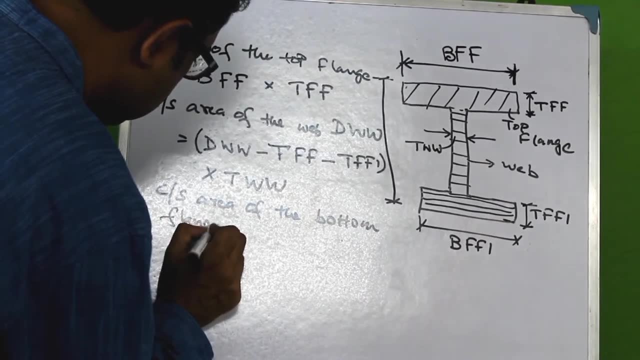 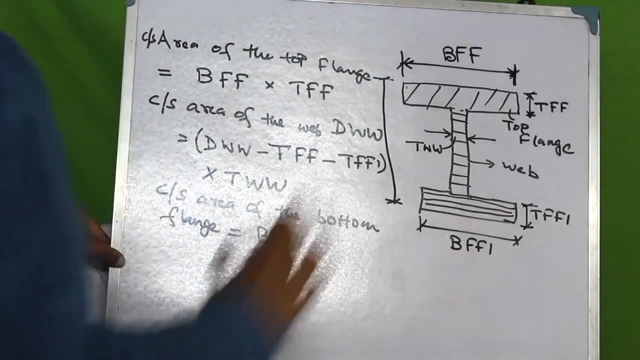 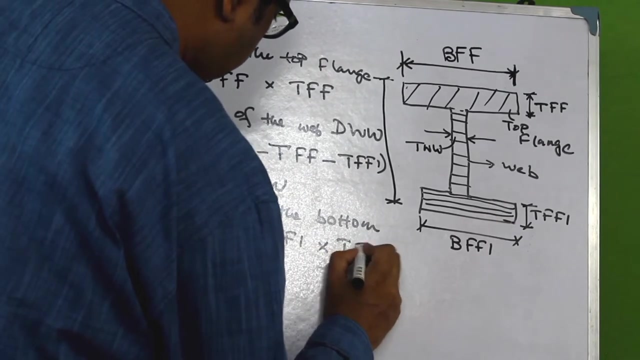 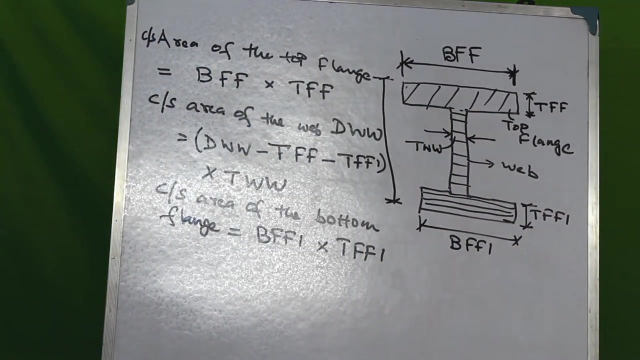 sectional area of the bottom flange, and this would be simply BFF1, which is the width of the bottom flange, multiplied by TFF1, which is the thickness of the bottom flange. so we have the cross-sectional area of all the three components of this particular section. so, therefore, the cross-sectional area of 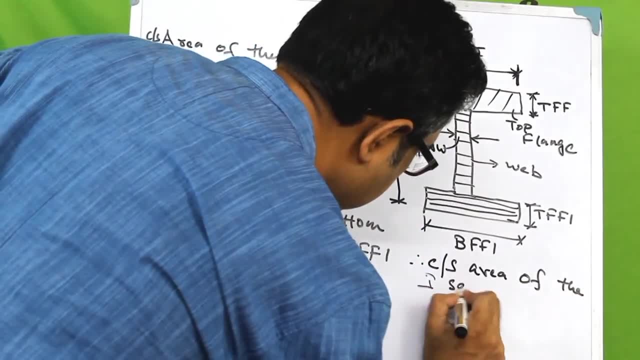 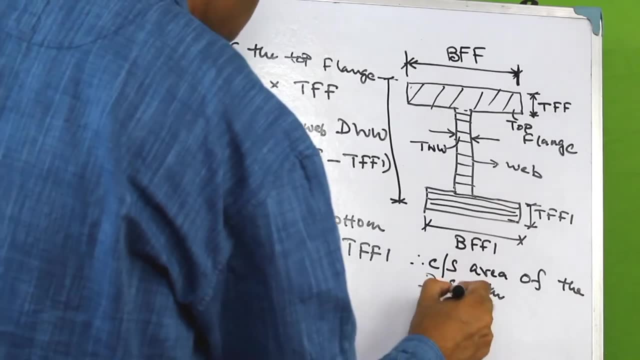 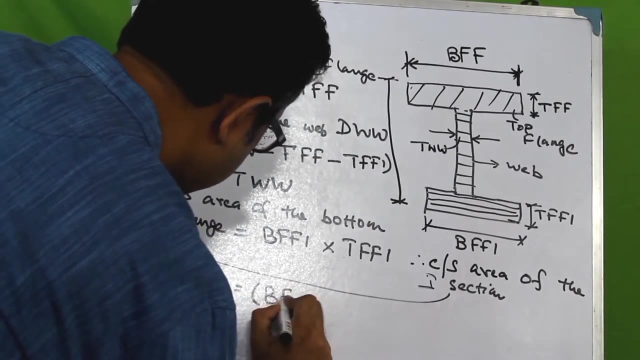 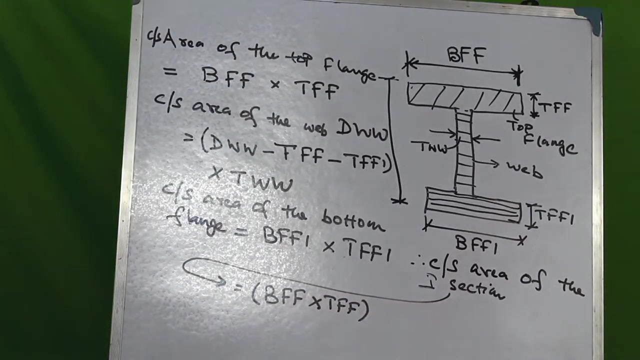 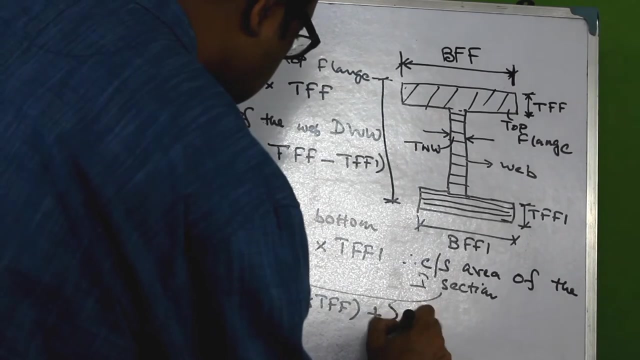 the I section will be the summation of all of this, so that would be equal to. so let us write from here. so it would be the first term in the expression BFF into TFF, which is the cross-sectional area of the top flange. then we have the second term, which would be now. this was: 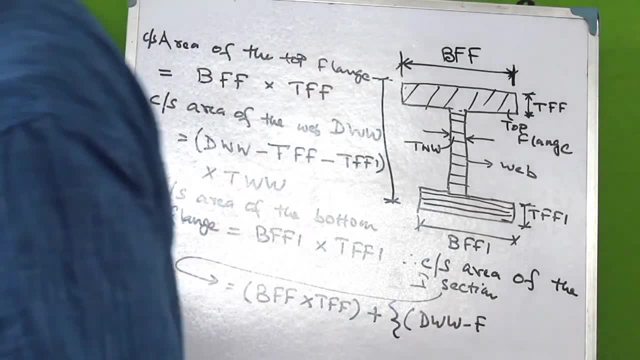 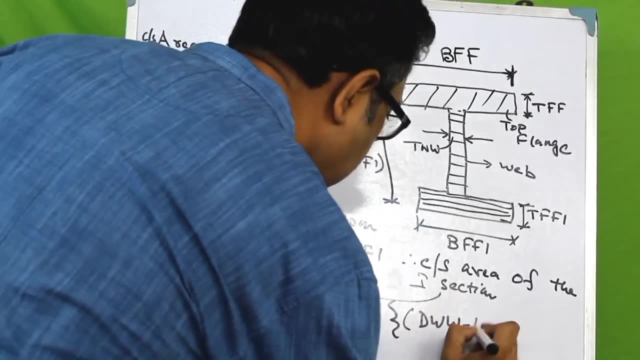 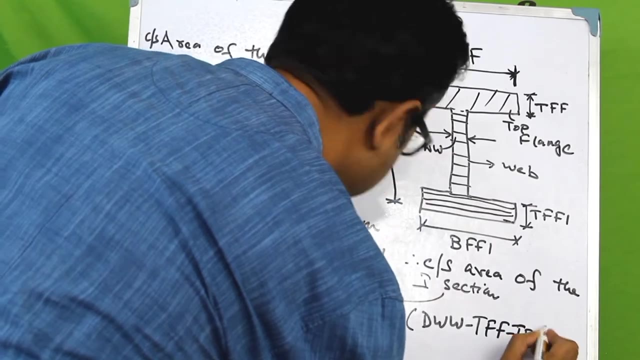 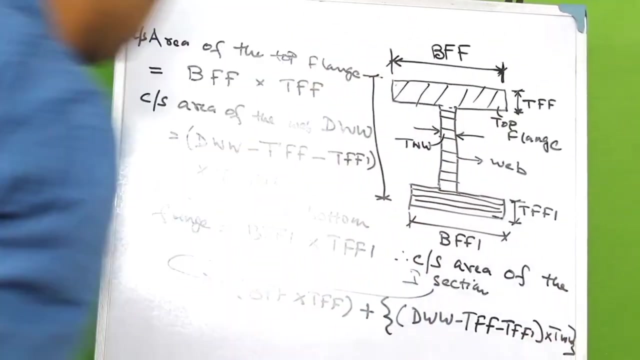 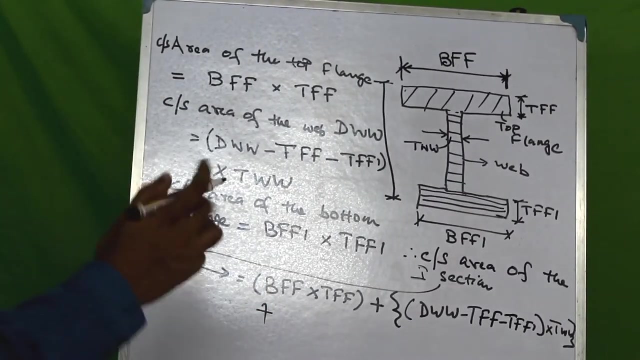 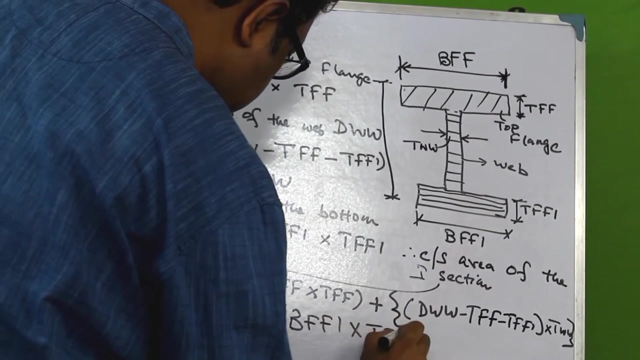 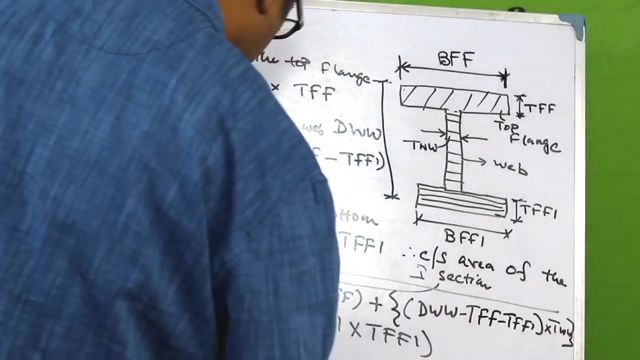 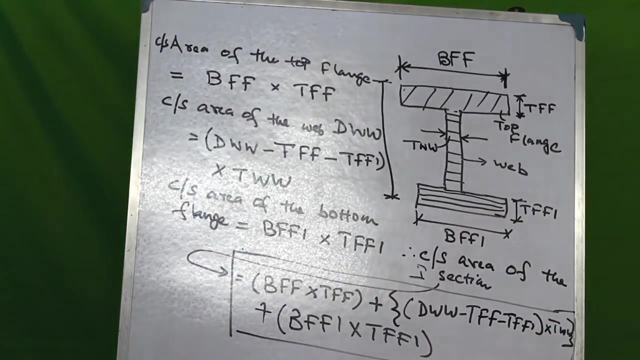 the depth, oh depth, of the web I Xэ, so bracket close. and finally the cross-sectional area of the bottom flange, which is pe0 V BF. so this, this expression here, gives you the cross-sectional area of the I section. now note that in most of the cases you would have the width of the the. 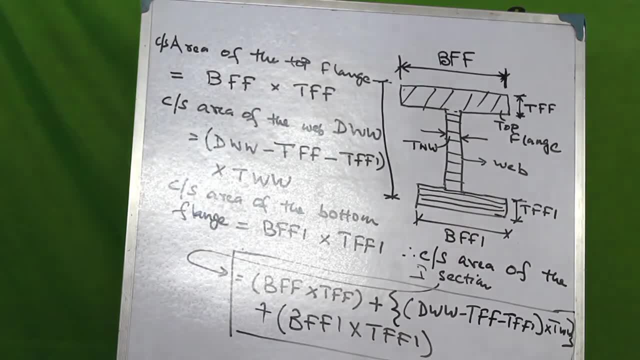 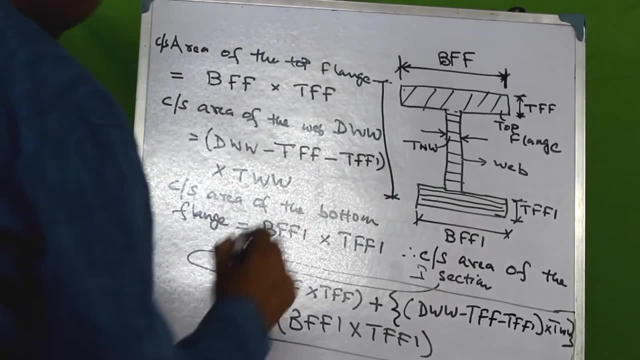 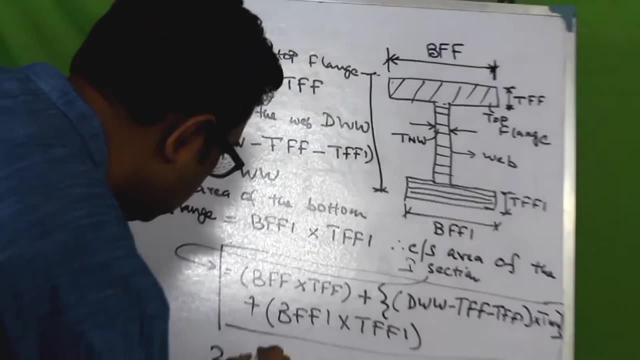 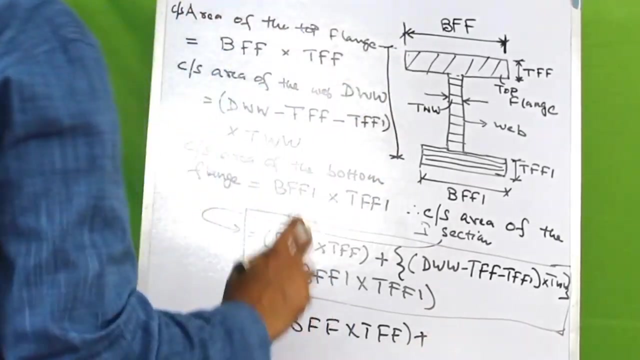 dimensions of the top flange, the dimension of the bottom flange, exactly the same. so in that case these terms would be the same. so in those cases you could represent this equation. so these two would be similar terms. so it would be 2 into and then this would be: 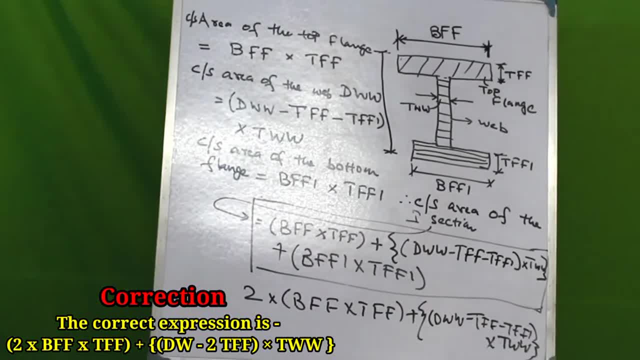 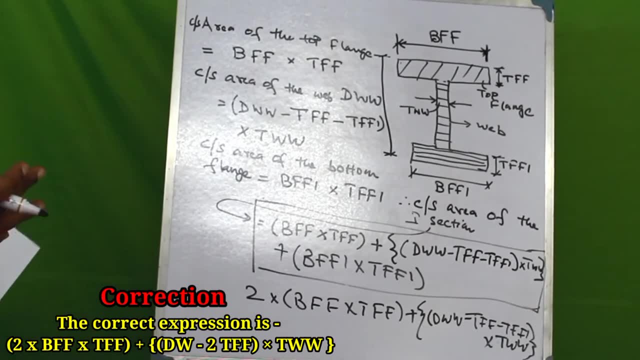 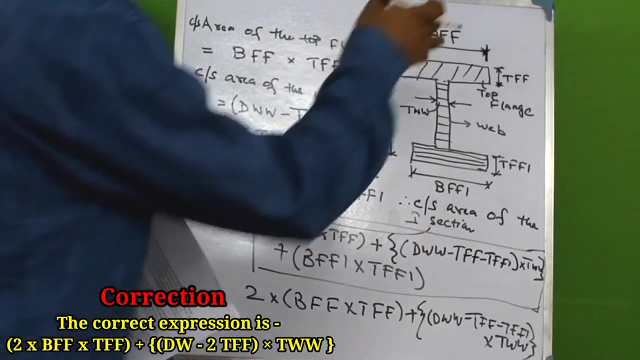 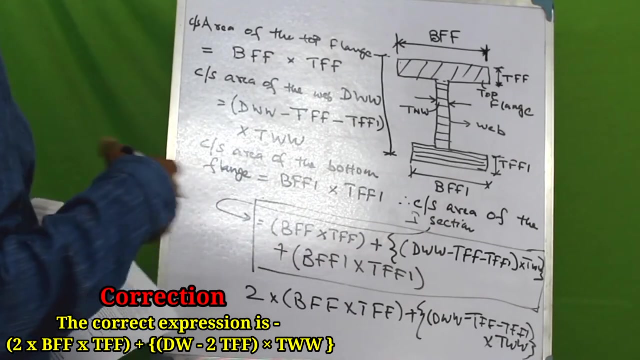 so now, one of the things that you have to understand is that the top and bottom are relative terms. now, in stat terminology those relates with the local axis of of the member. we haven't discussed the concept of local axis in a ZF, but we are coming to it, but the top and bottom in that case would be related. 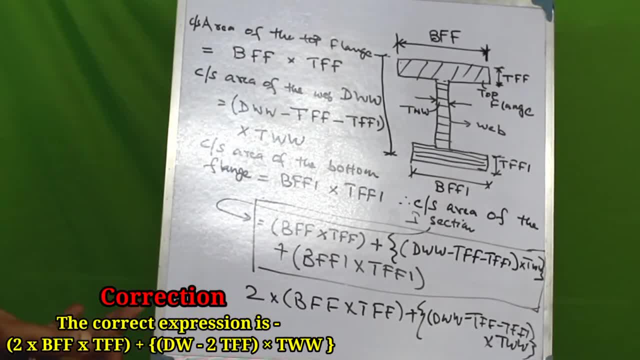 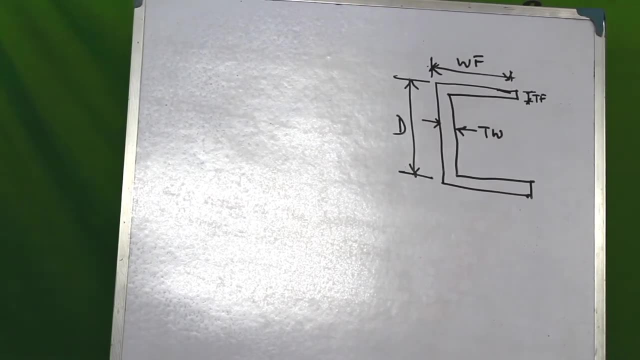 to the local axis of the number. okay, but we won't get into details into that. but for now just remember that there is a top flange and a bottom flange and that's purely a relative concert. so another type of sections that are available for still material is the channel section, which looks like this in: this case we have solid material, autologous Runner down, and then there are the connected sections, there's number and also the different dimensions that will rigned down. Am I doing this? well, transportation can be thezneata from this beat to machine, so we will be in contact. so the Kanal section is considered inter-channel sections in which we have these confirmed: no ratio in terms of theください of aberration. 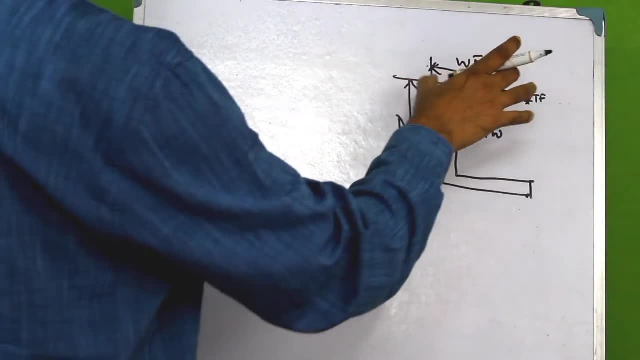 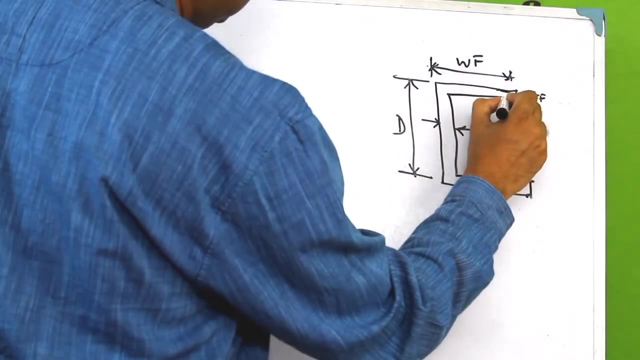 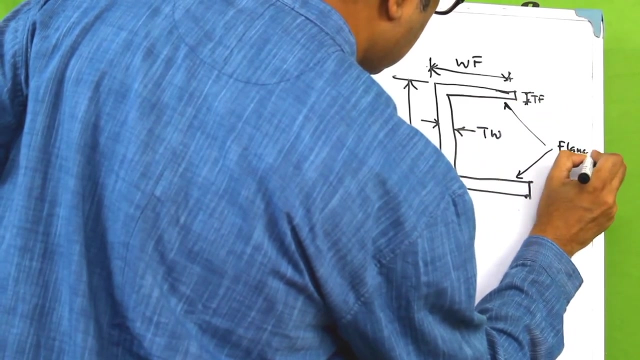 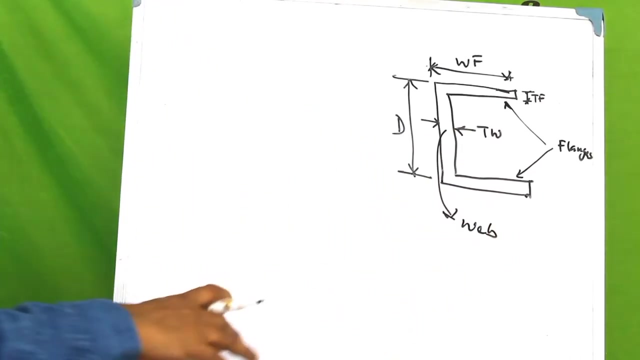 are assuming that, or generally, it so happens that the width of the flange for the top and the bottom flange of a channel section are exactly the same. Now, these are called the flanges for a channel section. So these are the flanges and this one is the web. Now, generally, 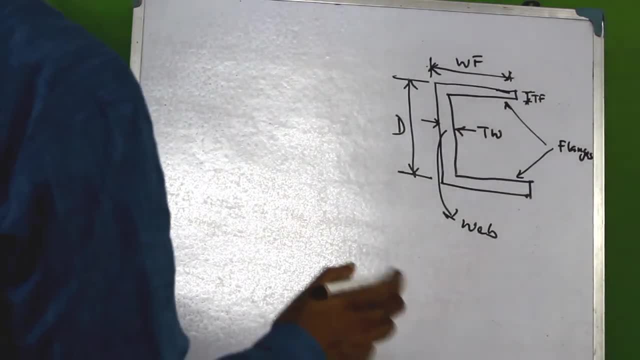 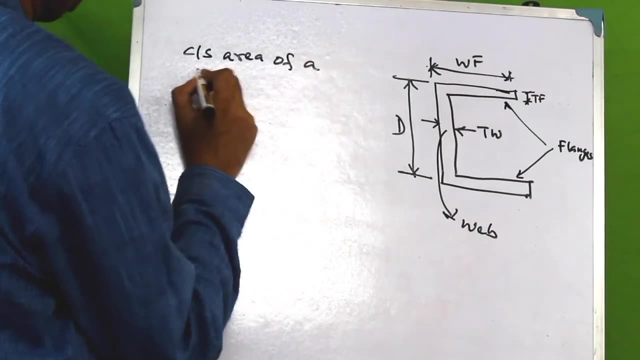 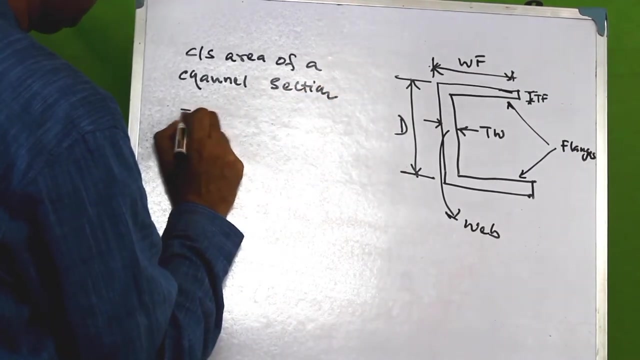 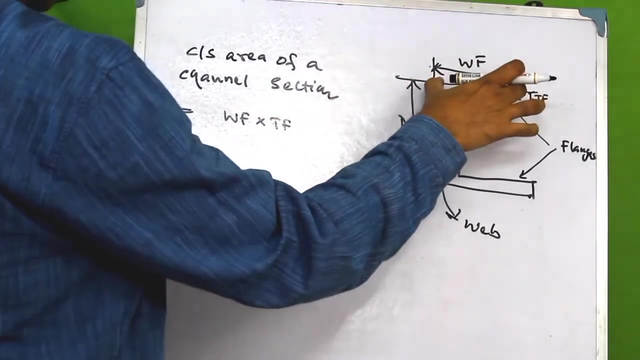 for a channel section. the width and the thickness are the same, So the cross-sectional area for a channel section would be calculated as so: this width of the flange into the thickness of the flange for the top flange. Now, exactly the same dimension is here. 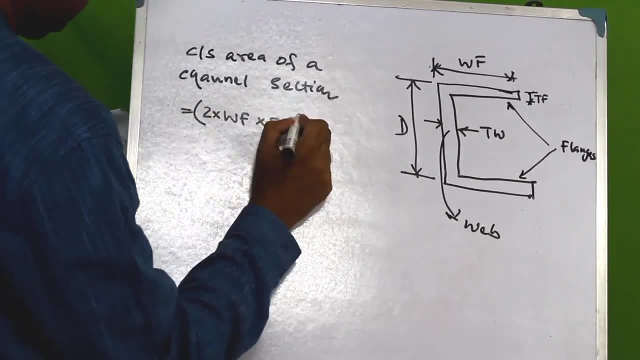 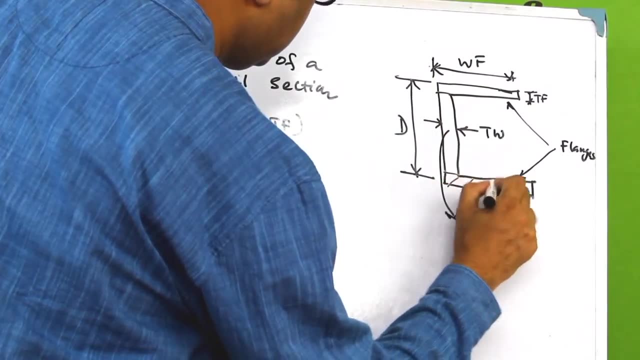 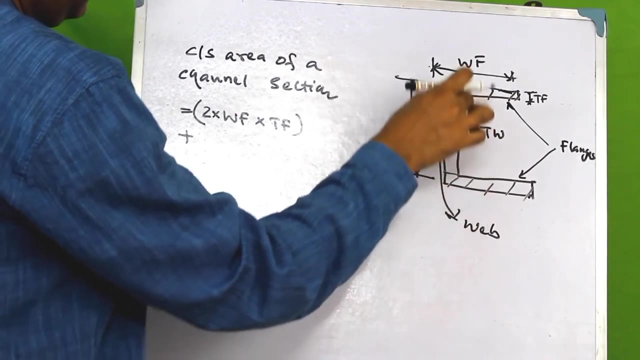 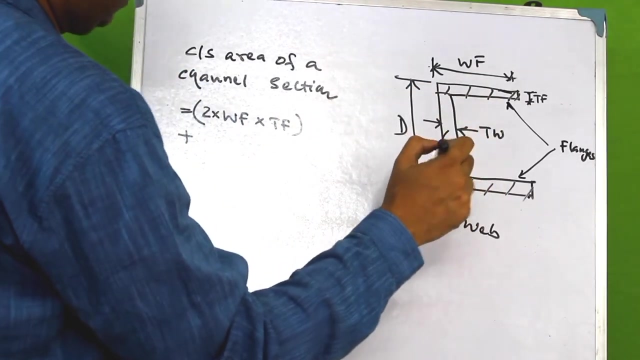 Right. So we multiply that by 2, like this, and the other component is the web. Now we have already taken the area of these parts, So only that remains is the area of this part web which is not shaded. So the depth then we have to consider would be the total depth minus the thickness of flanges. 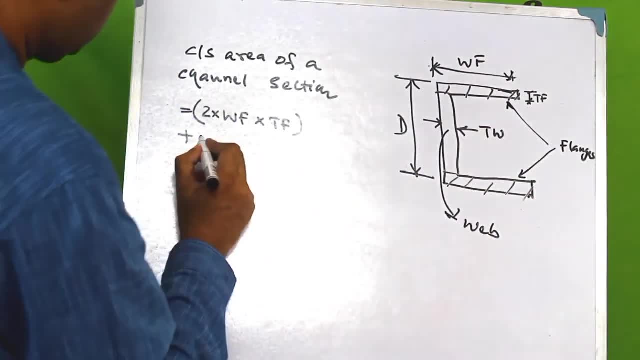 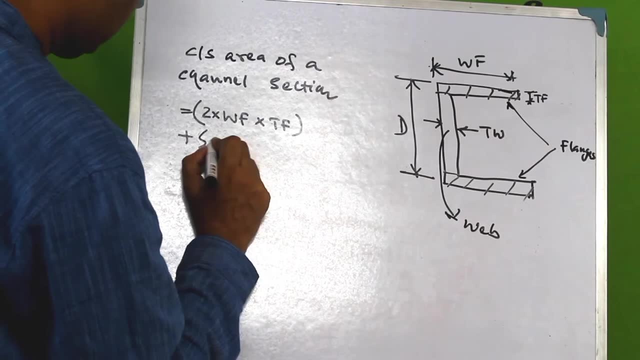 of the channel section. Now we have already taken the width, and then we have to consider the thickness of the flanges. Now the depth then we have to consider would be the total depth, the channel at the top and the bottom. so we will have the width. in this case is TW multiplied. 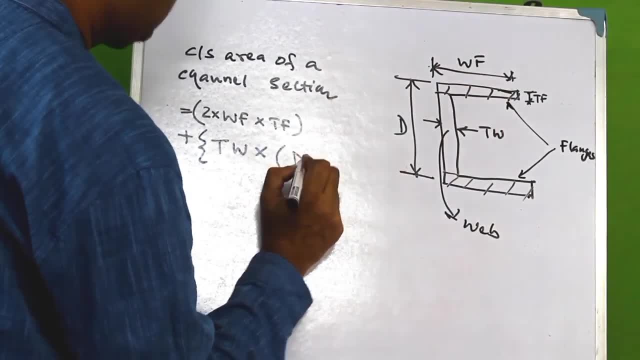 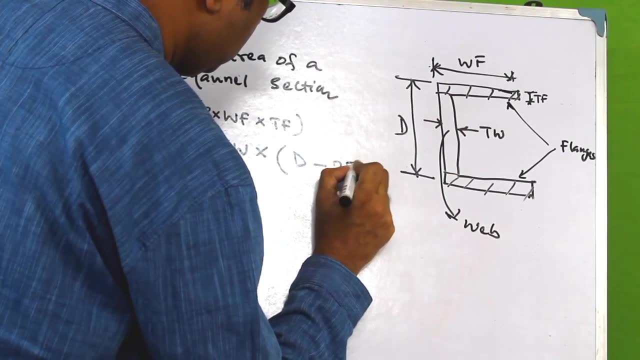 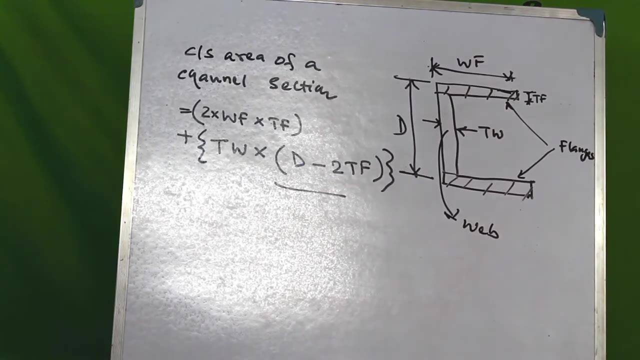 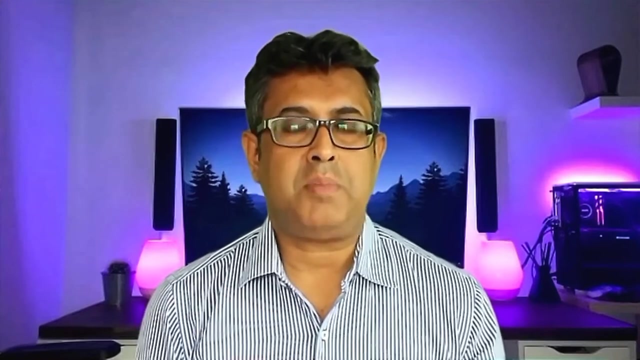 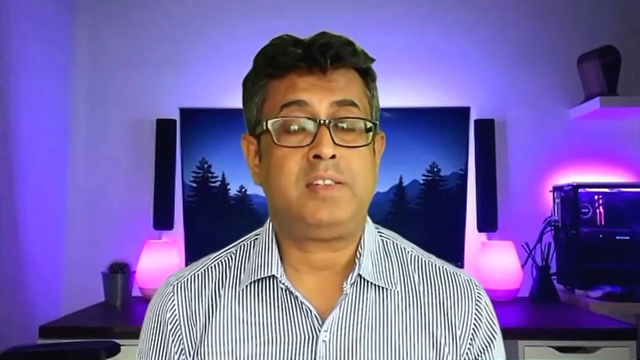 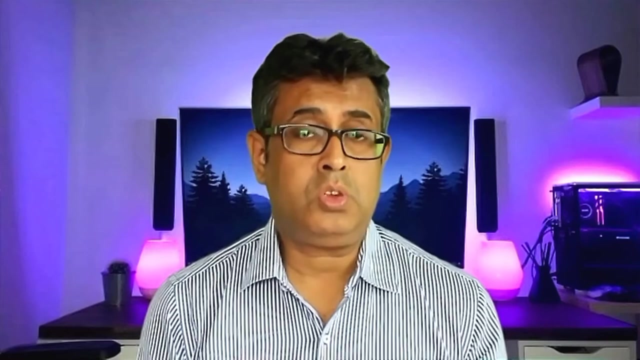 by this depth what would be given by G minus 2 into TF. so this is the cross-sectional area of the channel section. the terminologies that I have used to indicate the section dimensions are actually star crows way of representing sectional dimensions for the user-defined steel sections. now we will discuss in the future videos about the 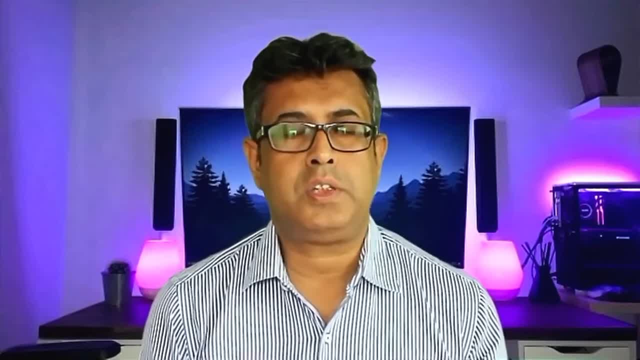 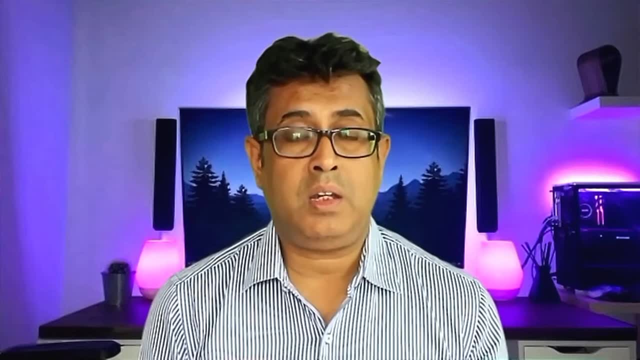 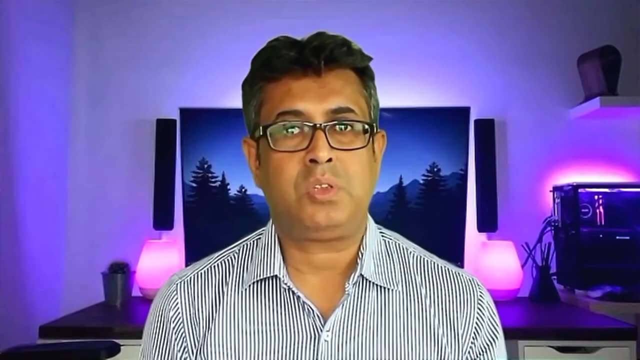 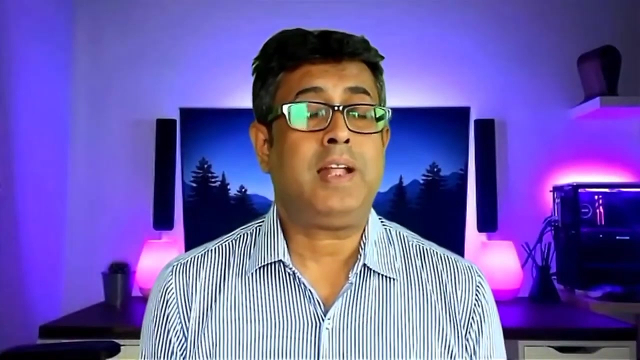 user-defined sections. user-defined steel sections in stat Pro. but one thing to note is that you do not actually need to calculate the sectional properties manually. once you specify the sectional dimensions for the user-defined steel sections, start automatically calculate the sectional properties. note that the cross-sectional areas of steel sections 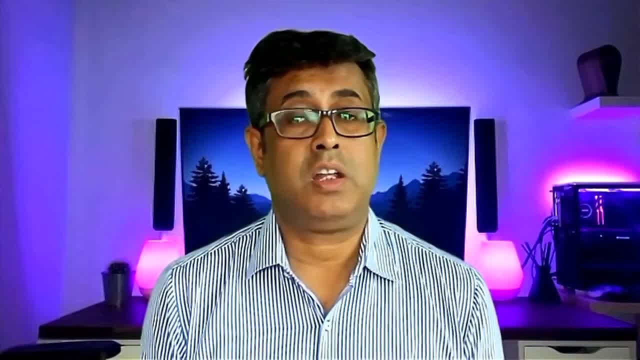 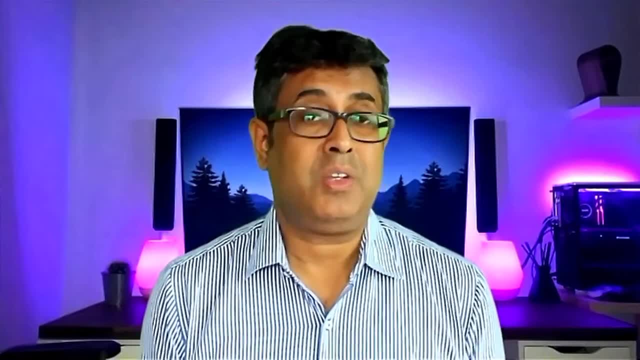 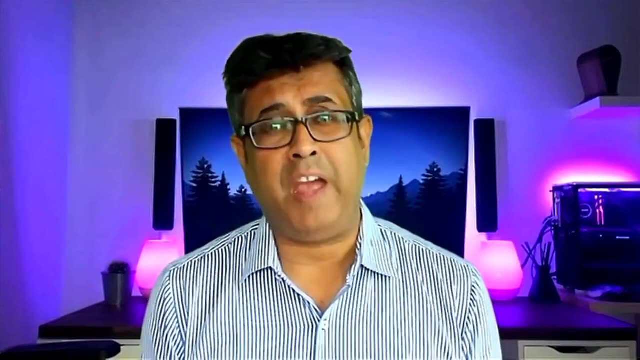 that would be rolled out of a factory, be it an I section or a channel section, will not exactly be the same as we had calculated using the rectangular components of the cross-section, because the sections that is rolled out of the factory doesn't exactly have rectangular section components. 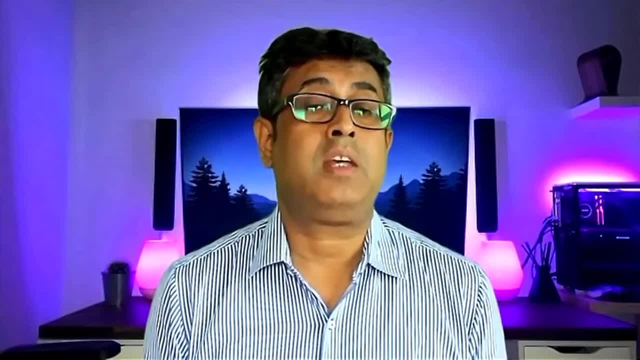 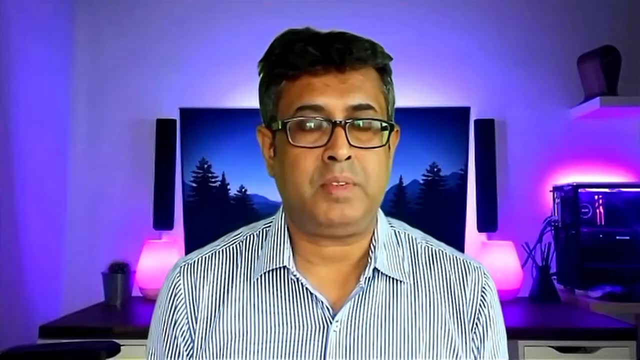 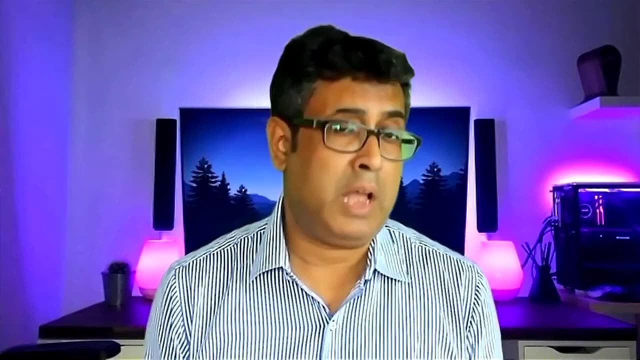 it has something called true videos, it is something called route ideas and they are on slopes in the section. if we use the rectangular approximation to calculate the cross sectional areas of those sections, there would be a degree of error in the cross-sectional area calculations. but we do not really.